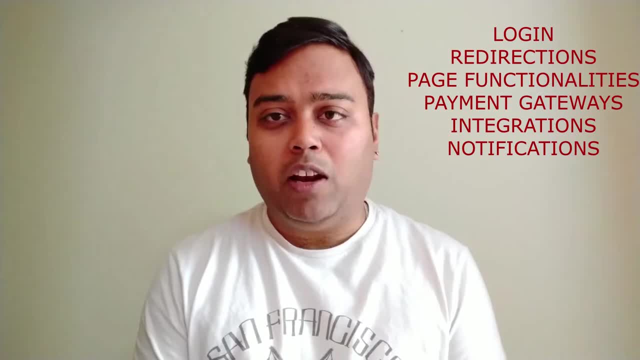 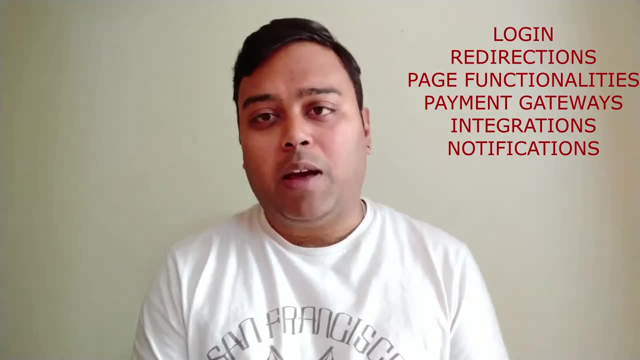 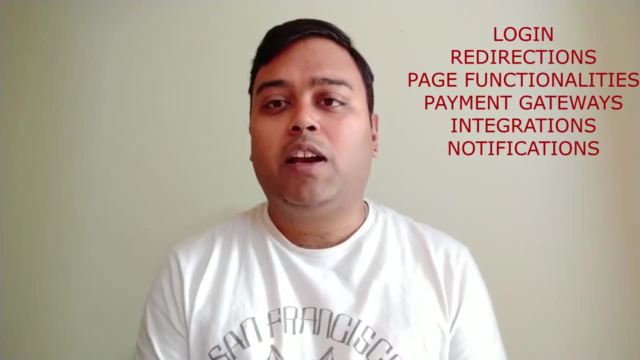 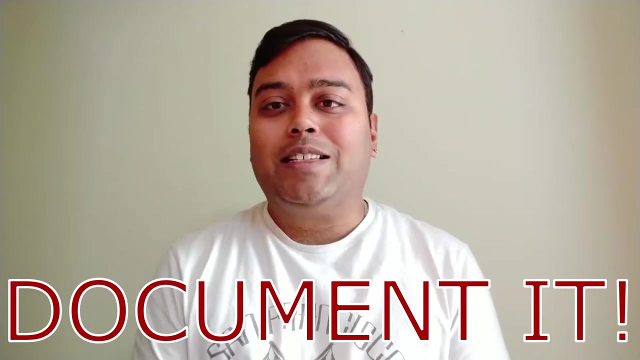 section which all payment gateways needs to be included, What is the information that needs to be gathered from the user and stored in the database, and things like that. The requirements at this stage should be very specific and should be documented with full carefulness. Otherwise, 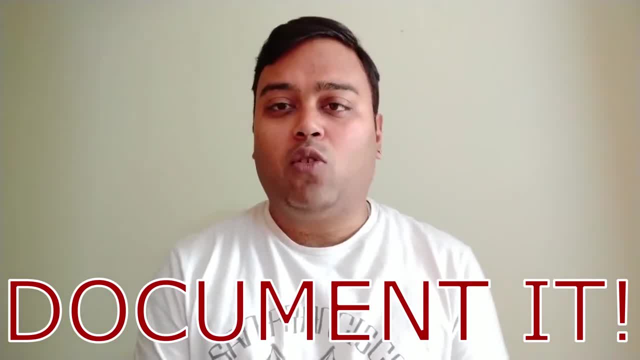 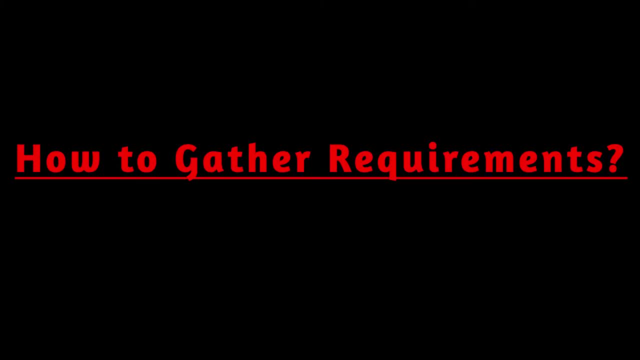 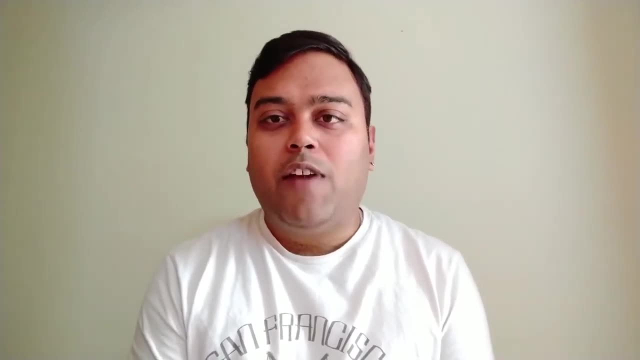 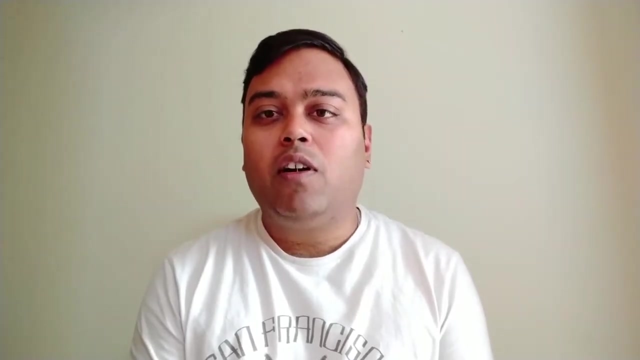 if there is an ambiguity left at this stage, it could create a problem for the developers while implementing them. Point is how to gather these requirements. Face-to-face interaction is considered the best way to gather the requirements from the client. However, the clients 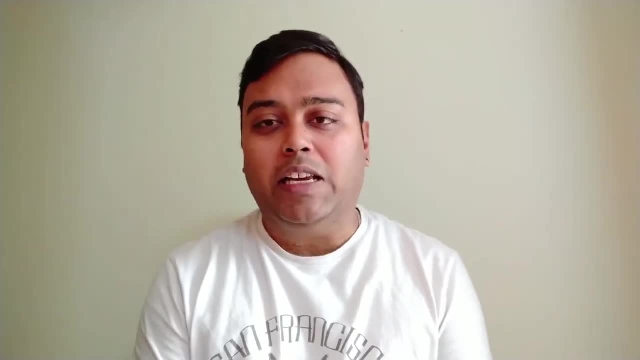 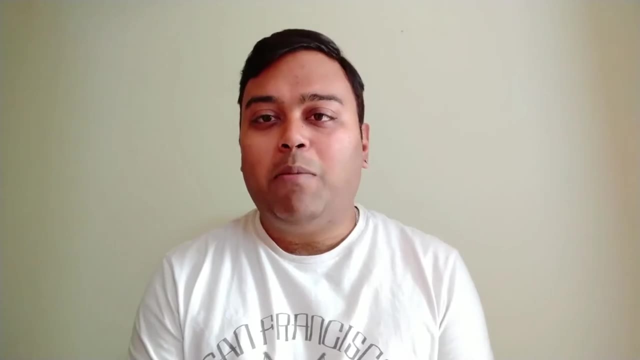 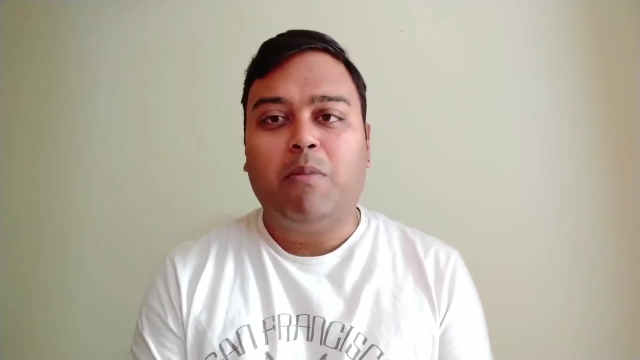 continue to stay in Europe, America, IE, Africa and few other places where it is difficult to travel. So online meetings through Skype Hangouts, GoToMeeting or times like these play important role where you could first meet face-to-face. face-to-face Because at the 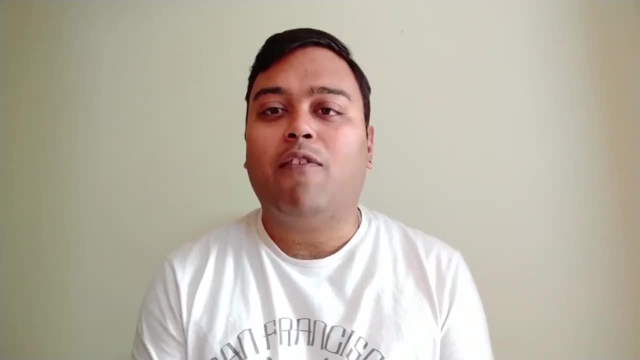 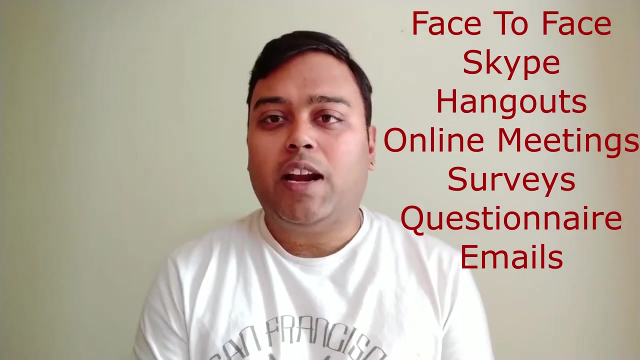 time of request, when the client answers, you could have an automating that allows you to ensure ensuring approval, Counter question or you could get those- your understanding- verified from the client. This is the fastest medium In case you cannot meet face to face. The other mediums are: you prepare a questionnaire and send it out to the client. 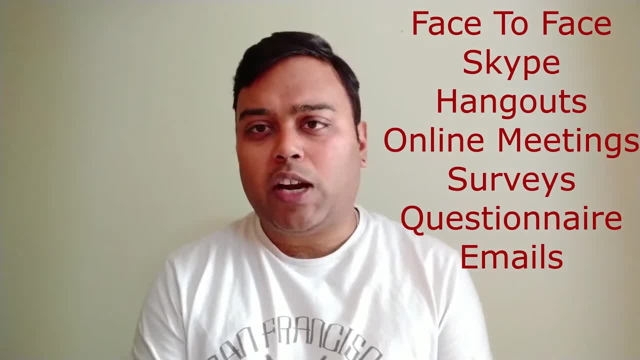 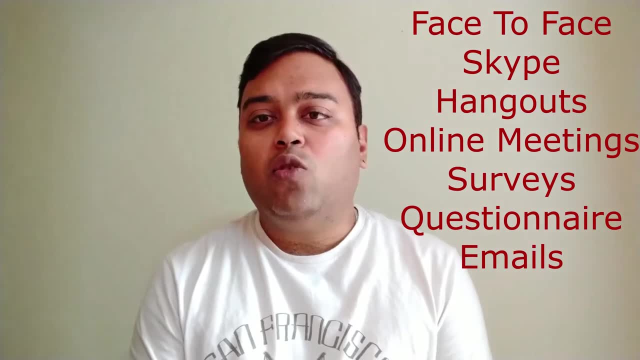 You prepare a sort of a survey and send it out to the client. or, lastly, an email is the best medium if nothing works, If the client is very busy, Then you can write down your questions or give them the options and ask them that how. please respond. 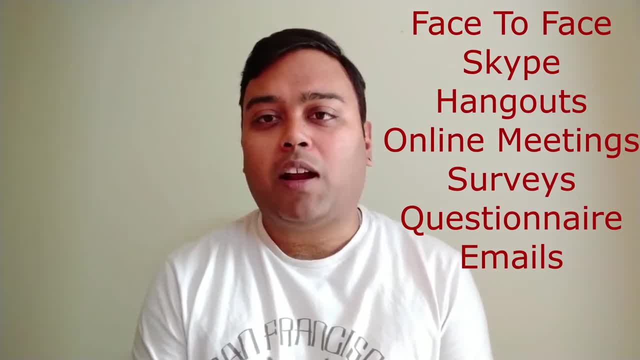 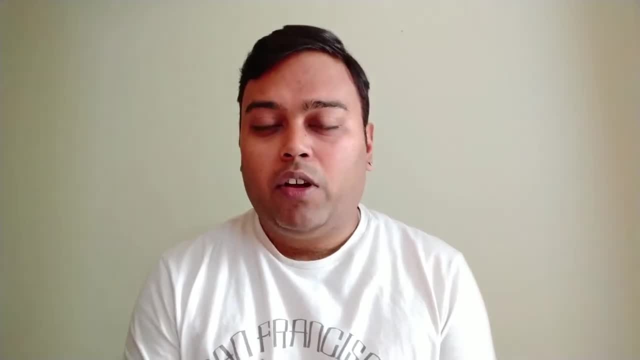 So these are the best mediums to gather the requirements from the client. Finally, verify the requirements. So you have multiple meetings with the clients. you have tons of emails coming back and forth. Now you have documented the requirements, But make sure that you verify With the client that is it what they really require or is it what they are looking for?